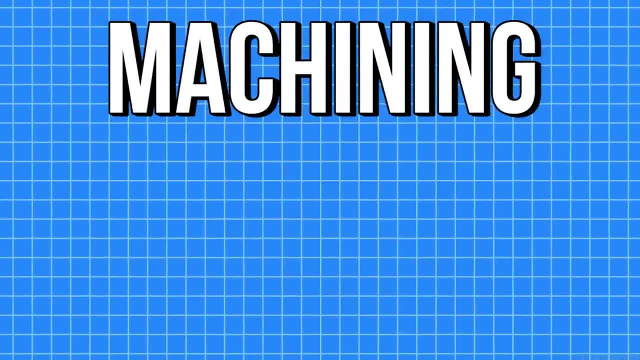 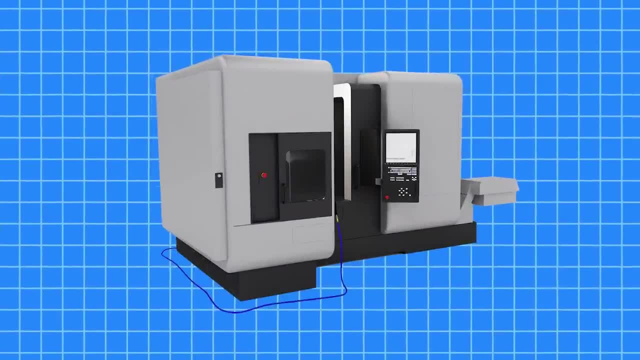 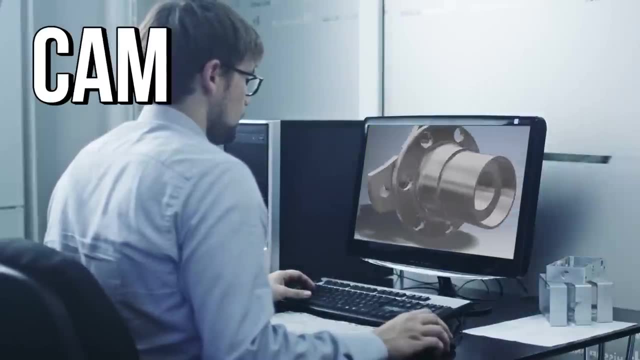 As mentioned before, machining is a way to transform a stock piece of material such as aluminum, steel or titanium into a finished product or part. CNC machines rely on digital instructions, specifically referred to as G-code, Before modern computer-aided manufacturing and computer-aided design programs, such as 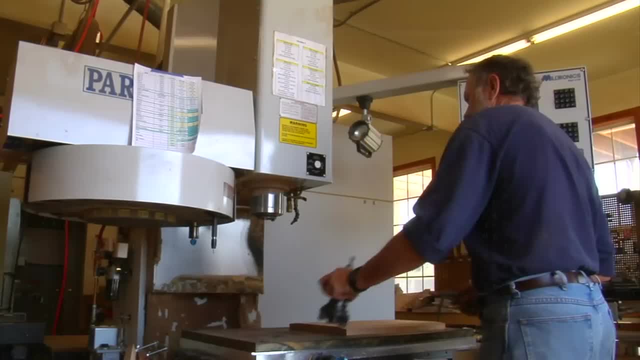 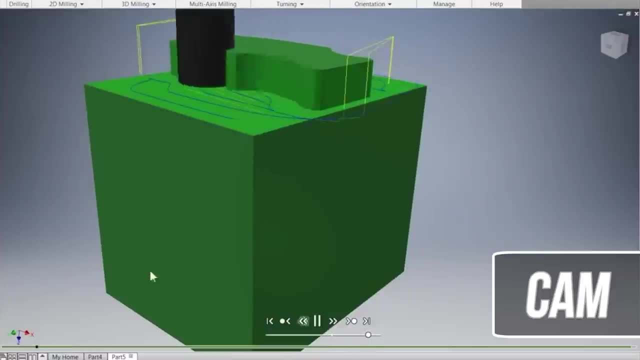 operating machines were developed. CNC machines were used for manufacturing and manufacturing. CNC machines were developed, specifically referred to as G-code. Before Autodesk's Fusion 360 were around, machinists would manually write the G-code to control these machines. CAM programs today allow you to take a 3D model and automatically generate G-code that. 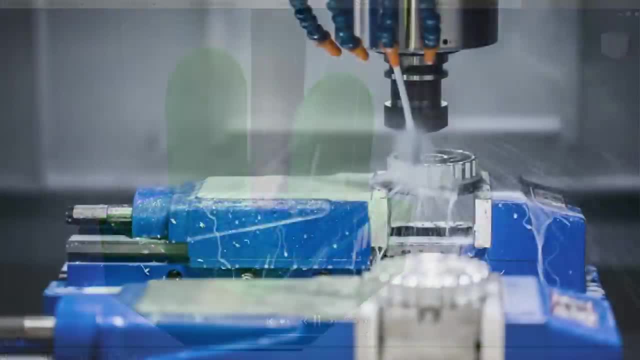 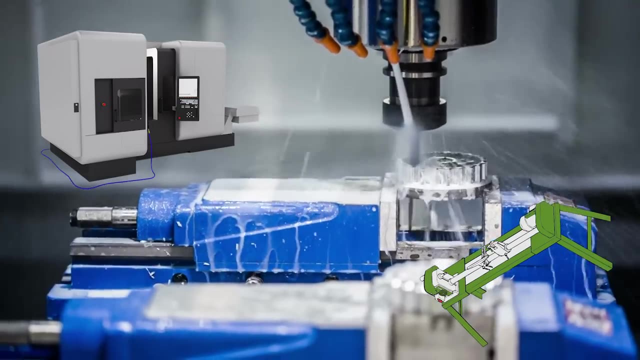 will drive the machine with little input. When you compare the capabilities of automated CNC machining to the manual alternative like lathes and other machining techniques, you can start to see the benefits. CNC machines simply run faster, at higher precision and accuracy, while simultaneously 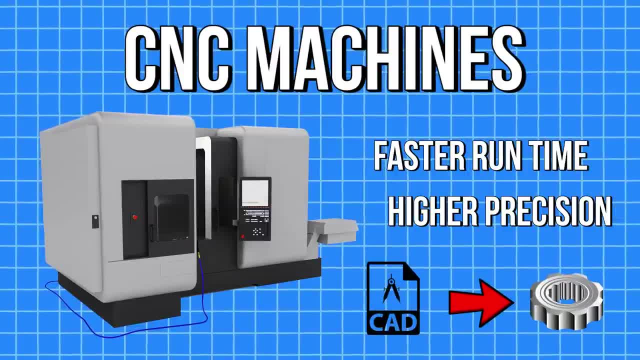 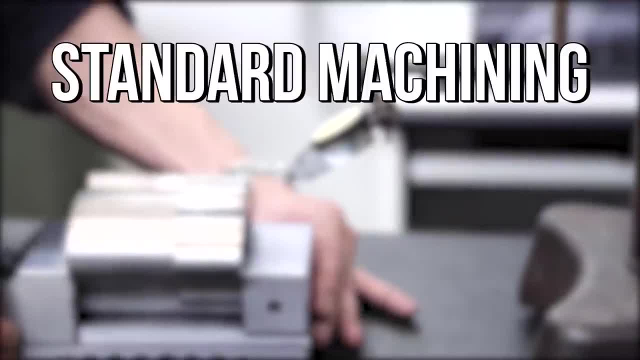 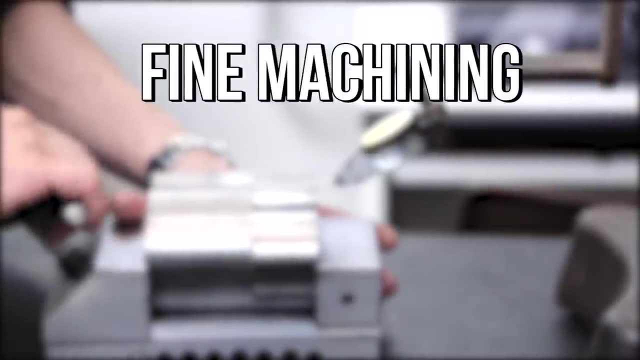 allowing the transformation of the machine. CNC machines are precise and are measured in thousandths of an inch, referred to as Thao. Standard machining can provide tolerances on parts around plus or minus .005 inches. Fine machining can produce tolerances of about plus or minus .001 inches and specialized 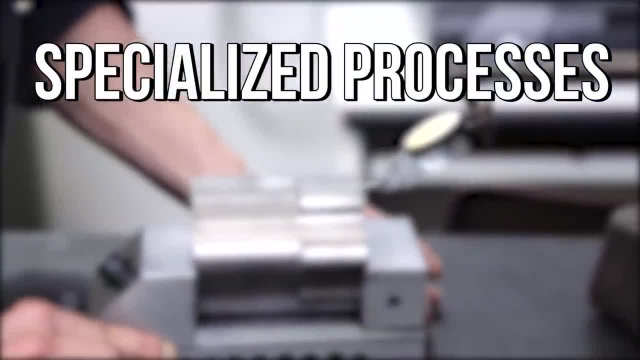 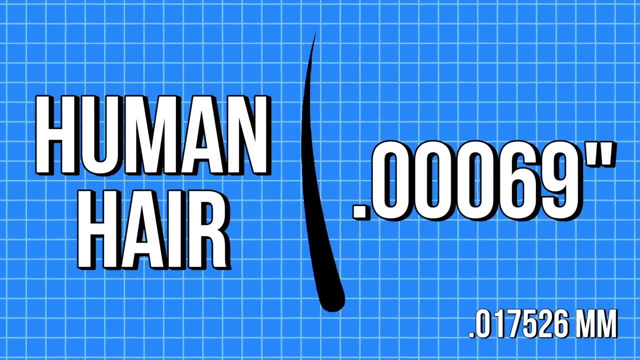 processes like polishing can offer up repeatable tolerances as tight as plus or minus .00005 inches. For reference, a CNC machine can be used for machining of parts around plus or minus .005 inches. For this, a human hair is .00069 inches thick. 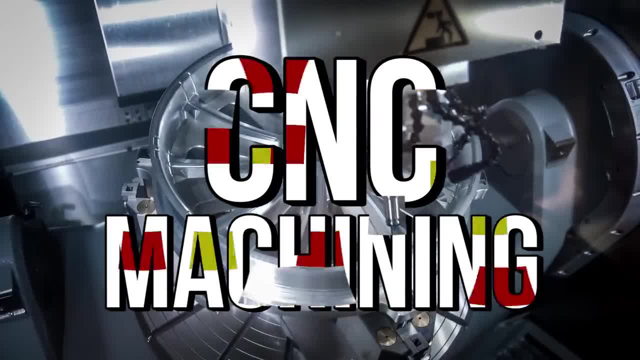 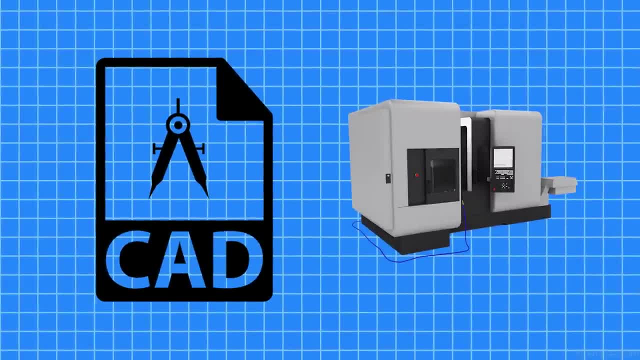 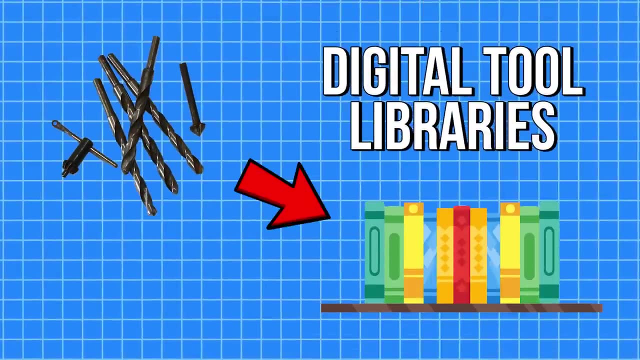 Now that we have the basics of CNC machining out of the way, we can start to dig into the intricacies held within. Many designs or specific machining processes require the use of multiple tools to make cuts. One tool doesn't function universally. For this, machinists will often build digital tool libraries that interface with the physical. 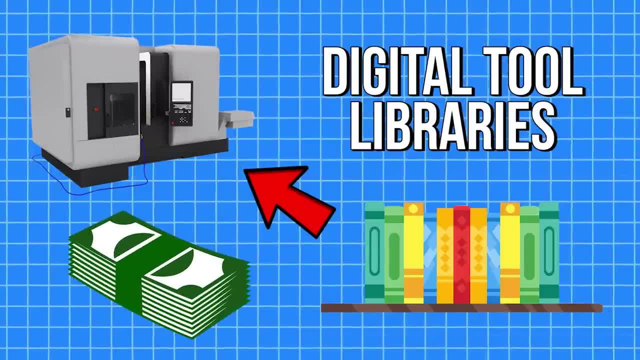 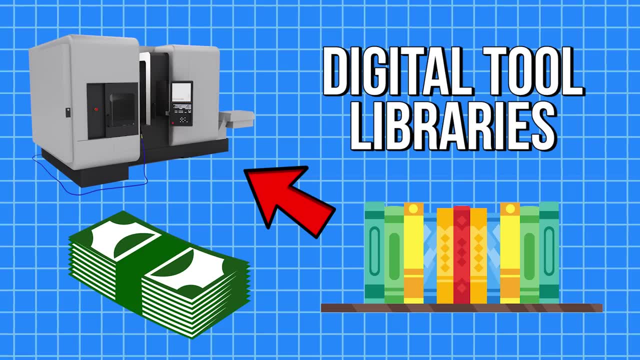 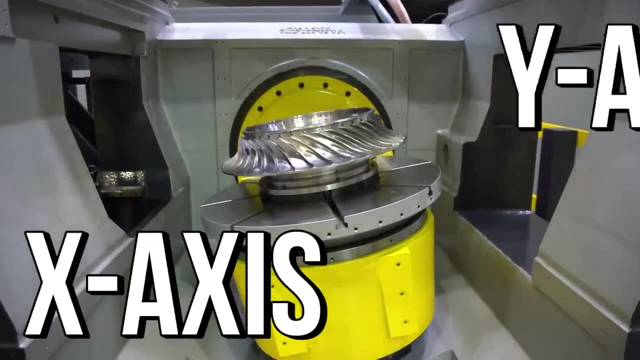 CNC machine. These machines, often costing hundreds of thousands of dollars, can automatically switch tooling when directed by their digital instructions, allowing for them to become manufacturing workhorses. Basic CNC machining will move one or two axes, referred to as the X-axis and the Y-axis. 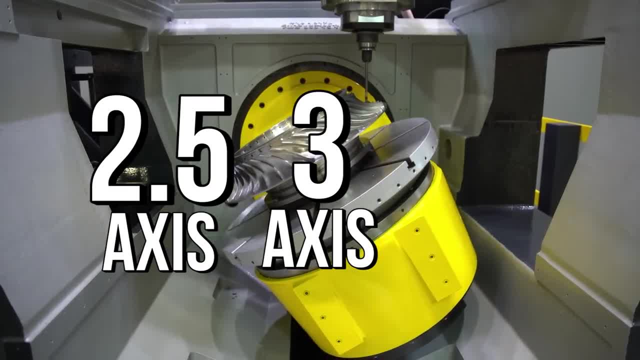 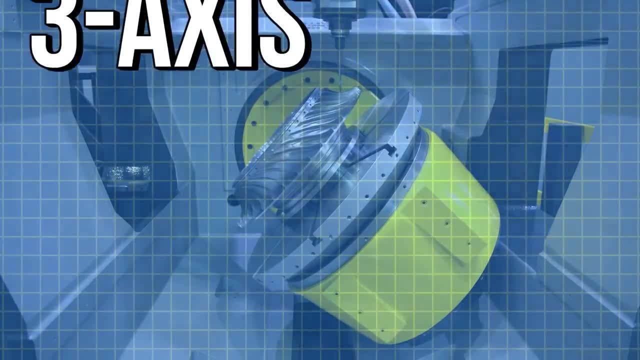 You'll often hear the terms 2.5-axis, 3-axis and 5-axis CNC machines, which simply refer to the degrees of freedom a machine can make cuts in. A 3-axis machine will move in the X, Y and Z-axis, whereas a 5-axis machine can move. 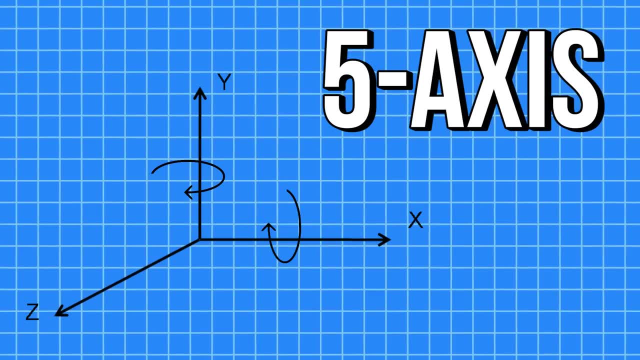 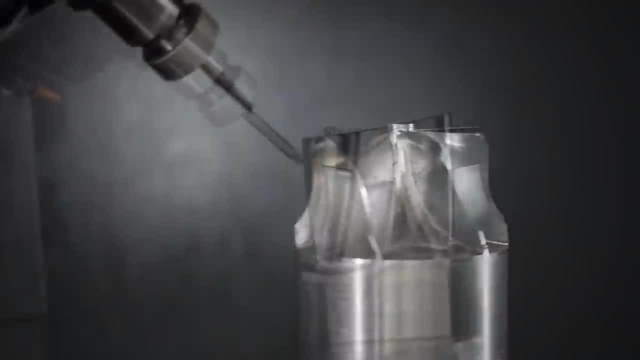 in the Y-axis, along with two additional rotational axes. As you might be able to imagine, the possibilities of production with 5-axis machines are practically endless. 5-axis machines used to be relegated to high-precision work, but as they have become more affordable, 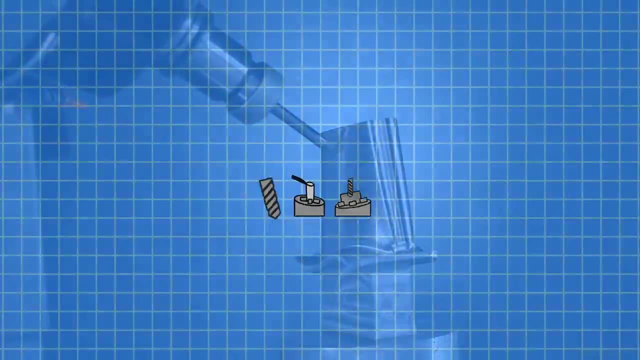 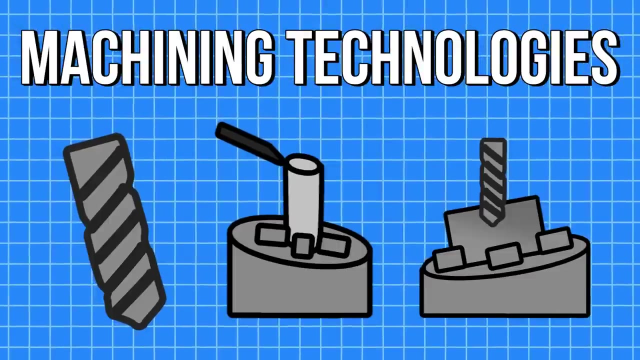 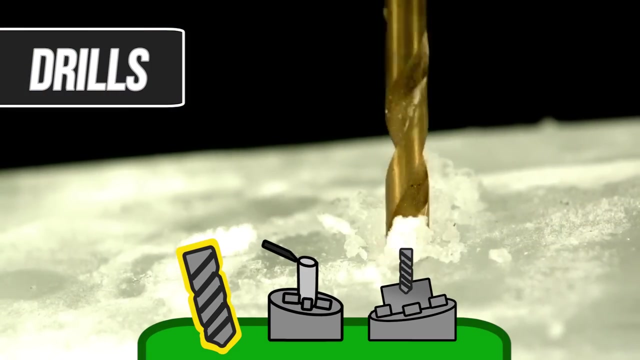 they are quickly becoming standard in many shops. There are three conventional machining technologies that you need to understand to grasp the basics of how material is removed from stock in CNC machines, The first being drills. Drills are the most common type of machining. Drills work by spinning a drill bit and moving a bit into contact with a stationary stock. 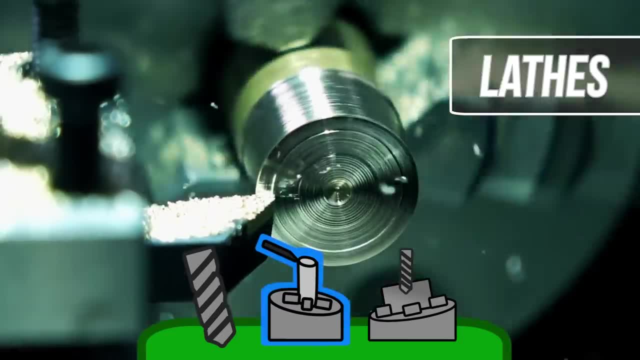 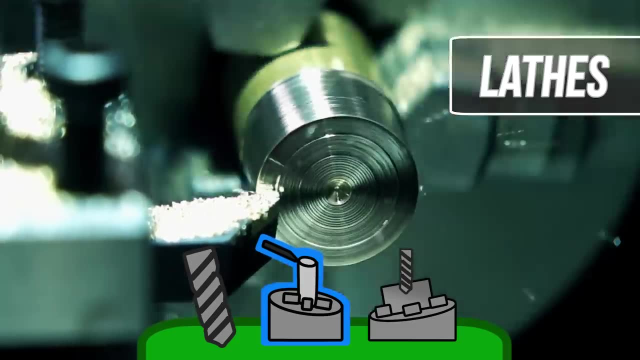 Next we have lathes which function in reverse to drilling. Lathes spin the block of material against a stationary drill bit or cutter to remove material in a circular or fluid path. The shape capabilities on lathes are more limited than other techniques, but modern. 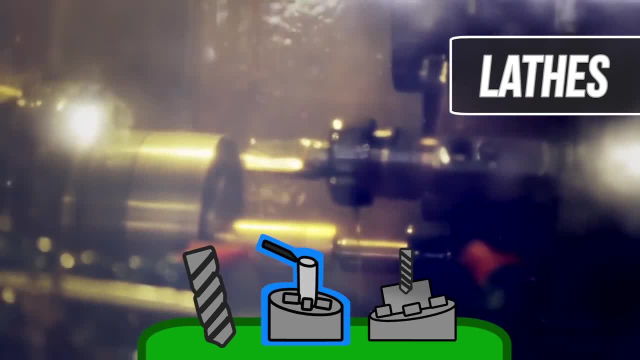 technology does allow these machines to create things such as square holes or non-circular shapes. Lastly, the most common CNC machine type is referred to as the 3-axis machine. which is referred to as the 3-axis machine. The 3-axis machine is the most common type of machining in CNC machining. 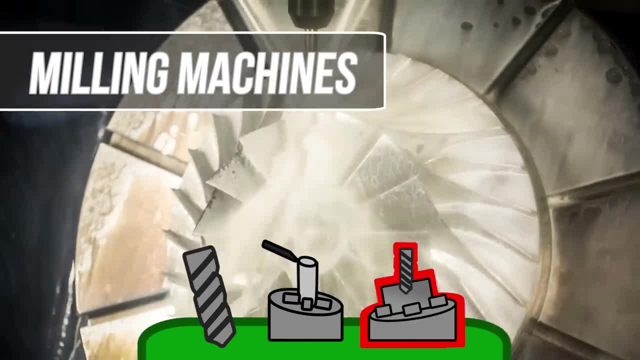 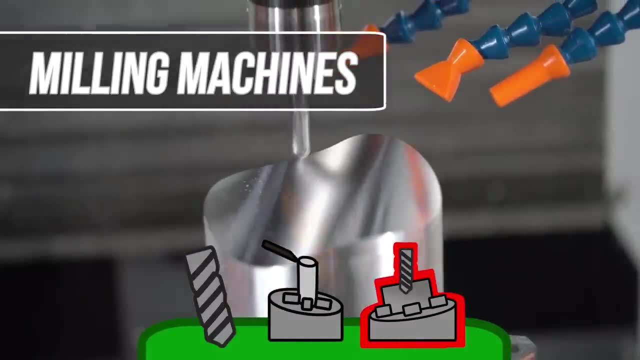 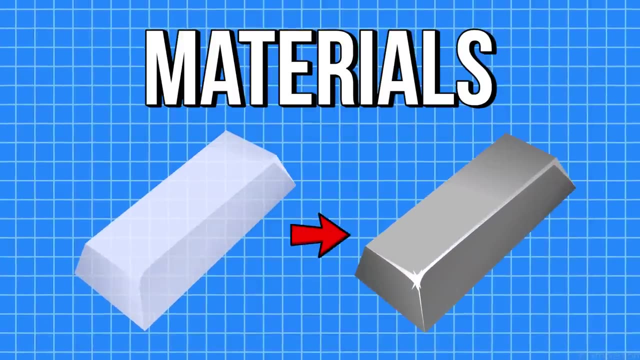 It is referred to as a milling machine. Milling machines involve the use of rotary cutting tools to remove material from a stock piece. These machines function similar to drills, with their tooling capabilities encompassing much more variety. Almost any material can be used in CNC machines, from plastic to titanium. 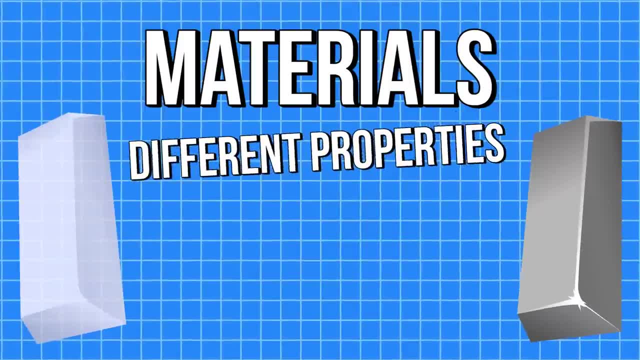 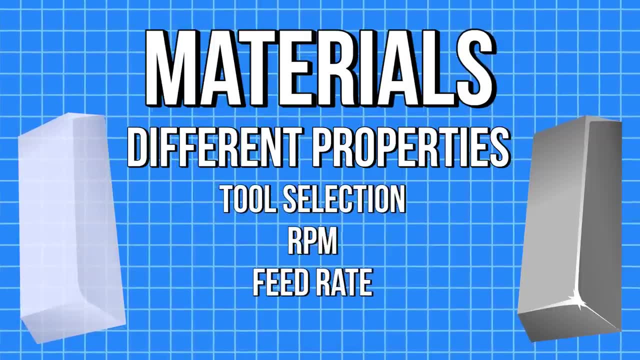 Different materials have different properties, so machinists and engineers will overcome their unique challenges by altering machining variables like tool selection, RPM, feed rate and coolant flow, among an extensive variety of other factors. CNC machined parts are all around you. 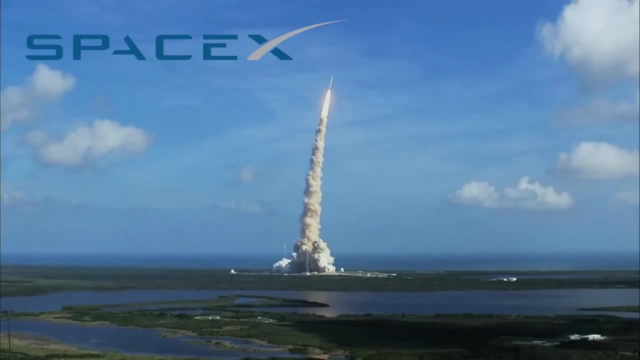 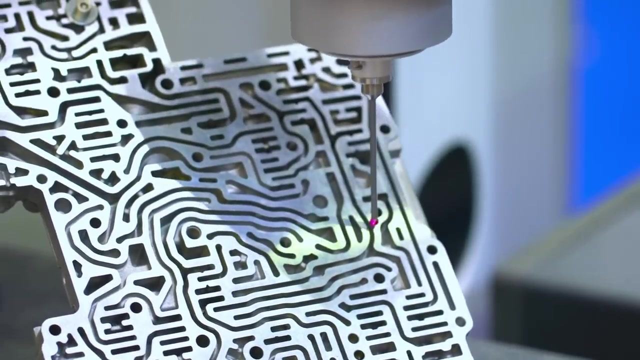 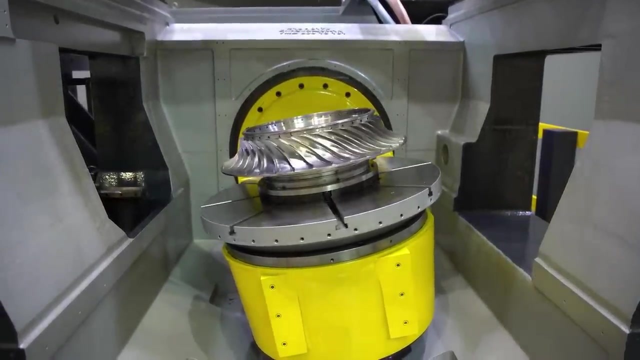 They hold together your car and perform vital functions aboard SpaceX rockets. CNC machining is arguably the only way to produce high-precision metal parts for engineering designs across the world. If you're interested in learning more about CNC machining and the crucial trade that it is, one of the best places to do that is through the titans of CNC Academy. 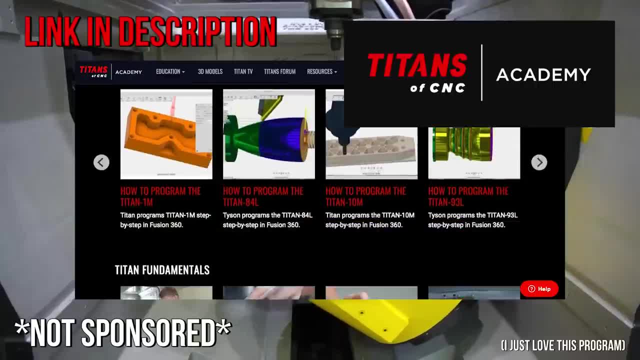 This online resource will take you to the best places to learn more about CNC machining and the crucial trade that it is. This online resource will teach you from the ground up how to design parts and machine them for free, whether you have a CNC machine or not.